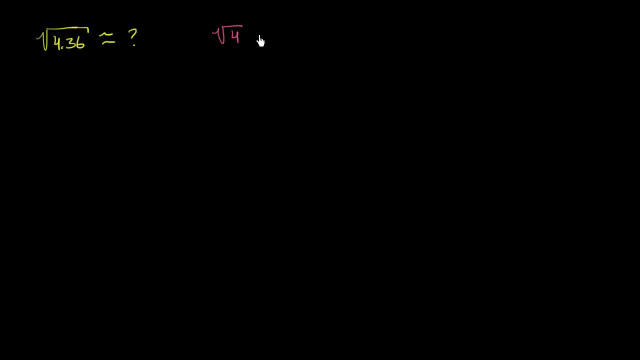 what the square root of four is. We know that this is positive two. The principal root of four is positive two. So you say, okay, this is gonna be a little bit more than two, But let's say that we want to get a little bit more accurate. 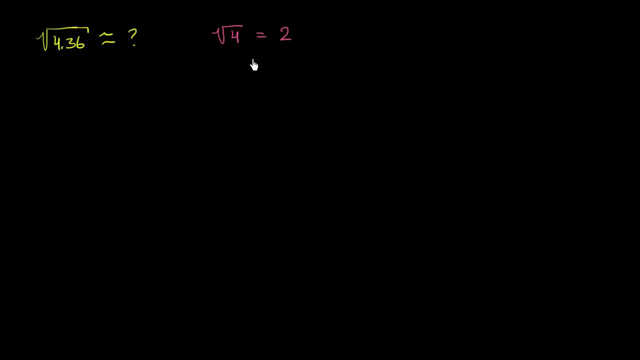 And so what I'm gonna show you in this video is a method for doing that, for approximating the value of a function near a value where we already know the value. So what am I talking about? So let's just imagine that we had the function. 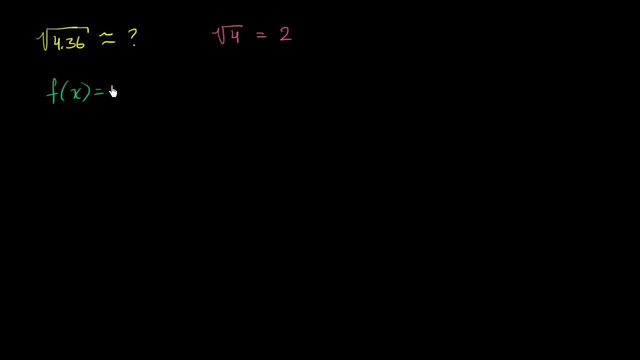 We have the function: f of x is equal to the square root of x, which is of course the same thing as x to the 1 1⁄2 power. So we know what f of two is. We know that f of two is positive two. 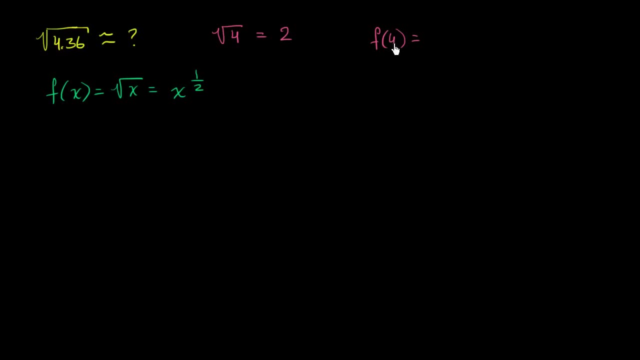 Sorry, we know that f of four is. We know that f of four is the square root of four, which is going to be equal to two, or the principal root of four, which is equal to positive two, And what we want to approximate. 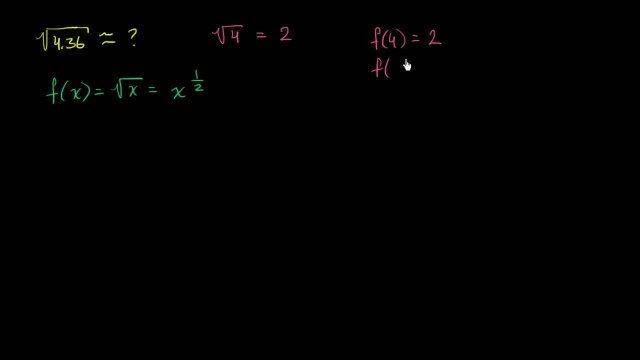 we want to figure out what f of we want to figure out what f of 4.36 is equal to. This is just another way of framing the exact same question that we started off this video. So let's just imagine our function. 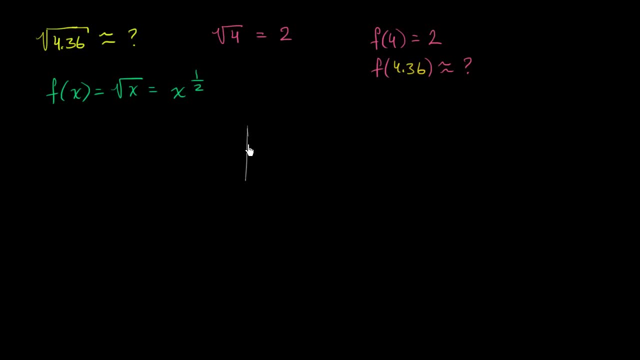 Let's just imagine it for a second. So let me draw some axes. This is my y-axis, This is my x-axis, And let's graph: y is equal to f of x. So let's say it looks something like this: Y equals f of x. looks something like that: 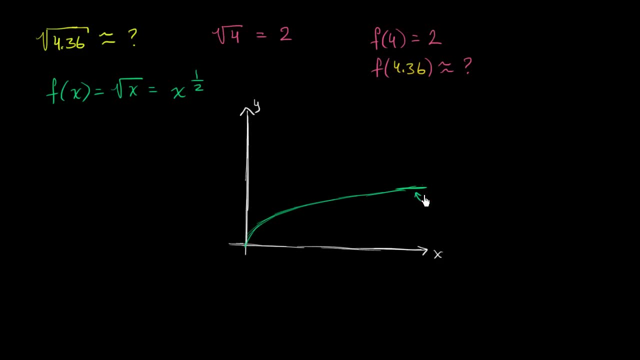 So that's pretty decent. All right, so that right there is: y is equal to f of x, F of four is equal to two, F of four is equal to two. So this is when x is equal to four. I haven't drawn it really to scale. 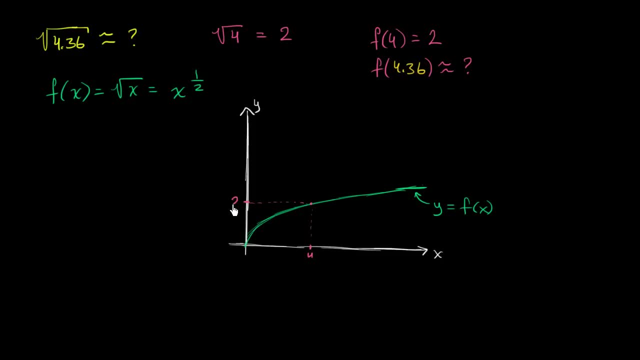 but hopefully this is clear enough, So that right over here is going to be two, That's f of four, And what we want to approximate is f of 4.36.. So 4.36 might be right around there And so we want to approximate this y value right over here. 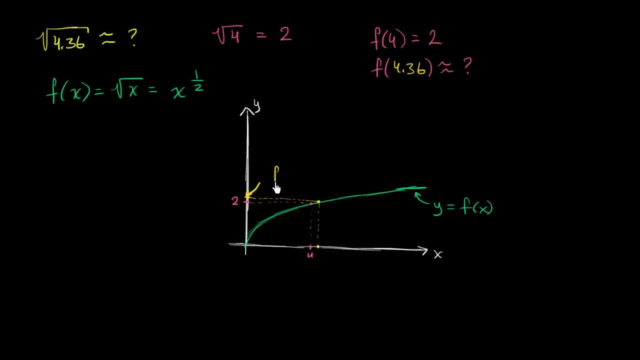 We want to approximate this y value right over here. We want to approximate that right over here is f of 4.36.. And once again, we're assuming we don't have a calculator at hand. So how can we do that using what we know about derivatives? 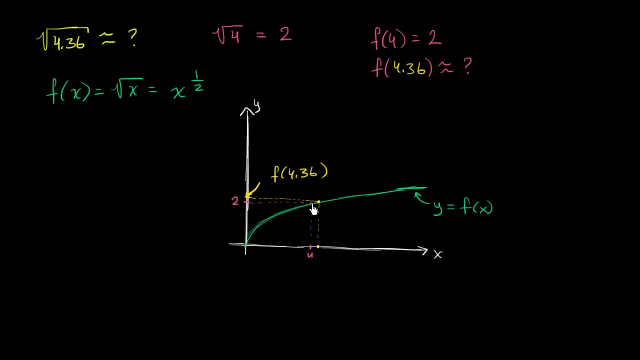 Well, what if we were to figure out an equation for the line that is tangent to the point, to tangent to this point right over here? So the equation of the tangent line at x is equal to four, And then we use that linearization. 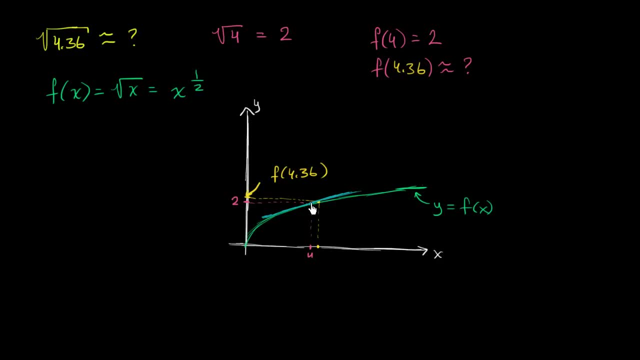 and then we use that linearization, that linearization to find, to approximate values local to it, And this technique is called local linearization. So what I'm saying is: let's figure out what the equation of this line is. Let's call that l of x. 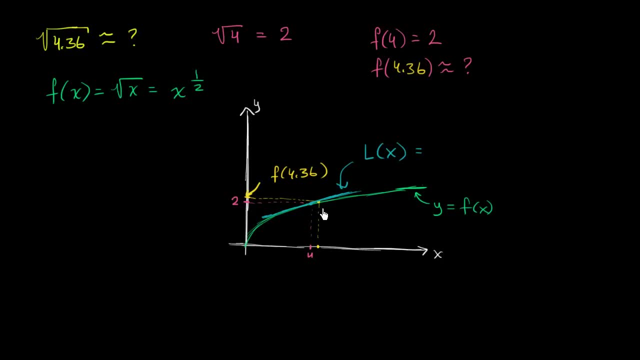 And then we can use that to. then we can evaluate that at 4.36. And hopefully that'll be a little bit easier to do than to try to figure out this right over here. So how would we do that? Well, one way to think about it. 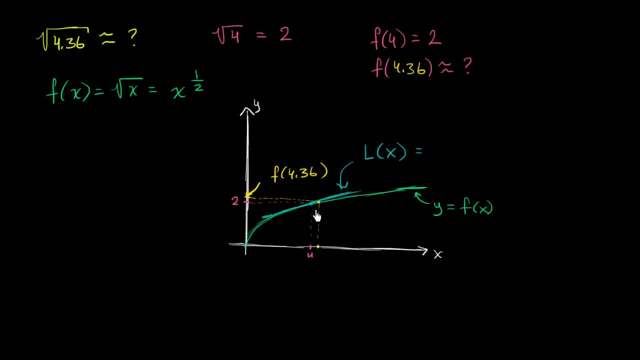 obviously there's many ways to explain this, There's many ways to express a line, But one way to think about it is: okay, it's going to. l of x is going to be, it's going to be. it's going to be f of four. 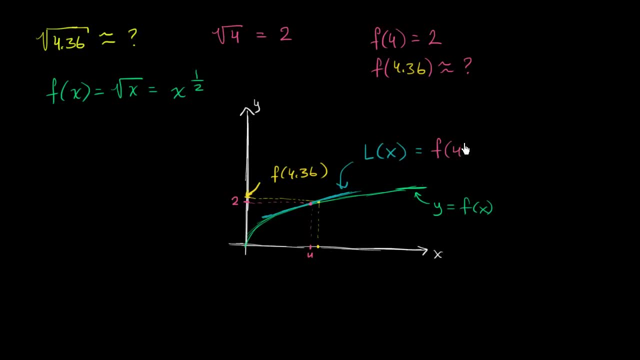 It's going to be f of four, which is two. It's going to be f of four plus the slope. the slope at x equals four, which is of course the derivative f prime of four. So that's going to be the slope of this line. 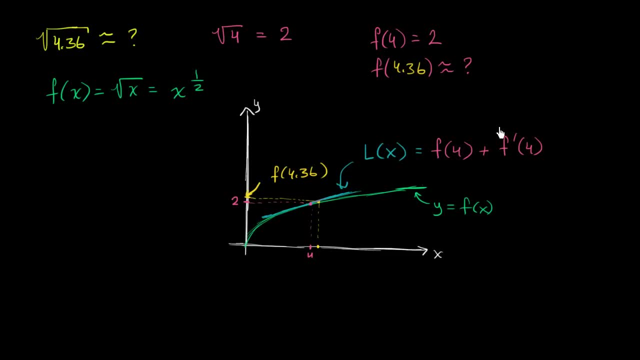 of l of x is f prime of four. Let me make that clear. So this right over here is the slope. the slope at x equals four, So it's the slope of this entire line And so any other point on this. it's going to be f of four plus the slope. 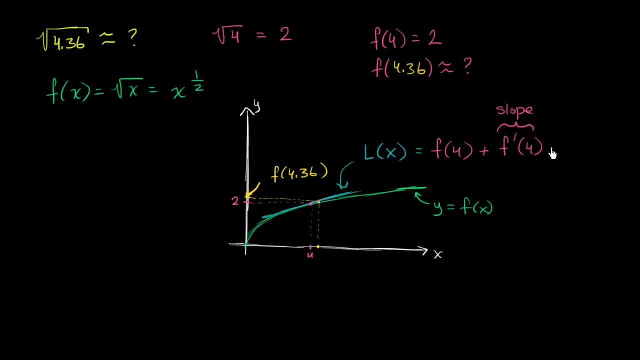 times how far you are away from x equals four, So it's going to be times x minus four. Let's just validate that this makes sense. When we put 4.36 here, when we put 4.36 here actually, let me zoom in on this graph. 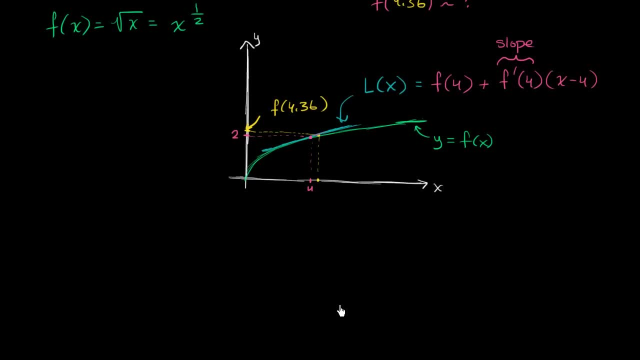 just to make things a little bit clearer. So if this is so, I'm going to do a zoom in. I'm going to do a zoom in. I'm going to try to zoom in into this region right over here. So this is the point. 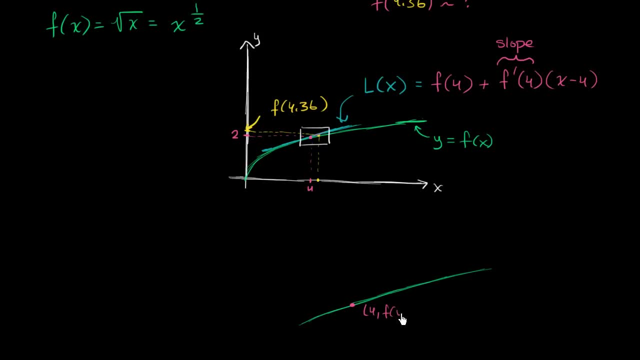 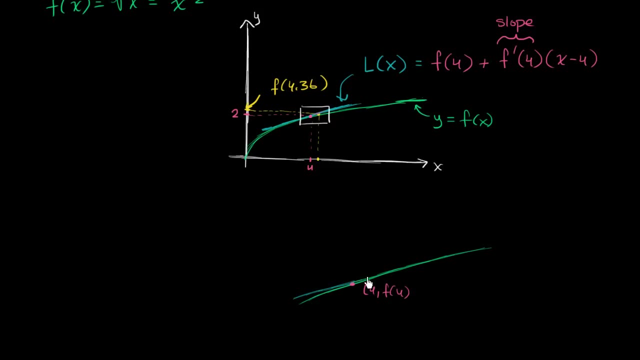 this is the point four, comma f of four, And we are going to graph l of x, So let me do that. So this right over here is l of x, That's l of x, And let's say this right over here: 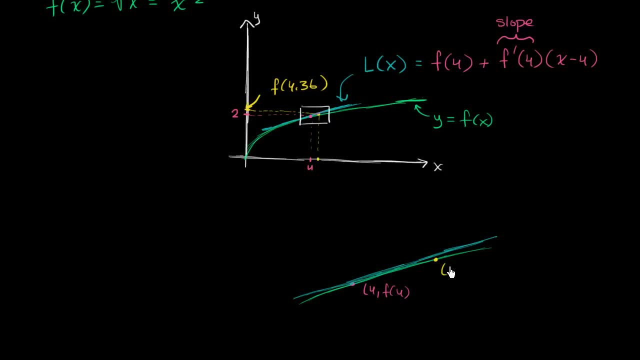 this right over here is the point 4.36, comma f of 4.36.. And the way we're going to approximate this value is to figure out what, to figure out what this value is right over here And what is this one going to be. 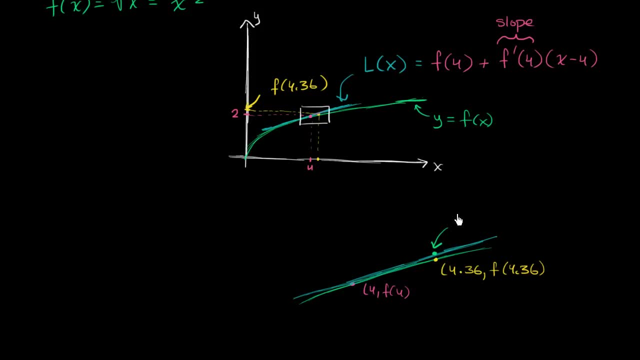 This right over here is going to be. this is going to be 4.36 comma l of 4.36.. This line evaluated when x is equal to 4.36.. And what is that going to be? What is that going to be equal to? 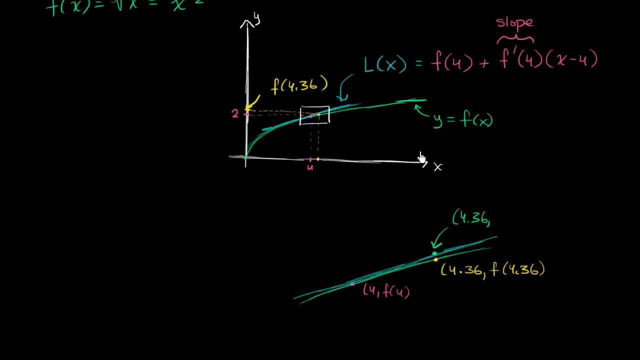 Well, let's see, let's just evaluate it. l of 4.36 is going to be f of 4.. So it's going to be 2 plus the derivative, so the slope of this line plus f, prime of 4. 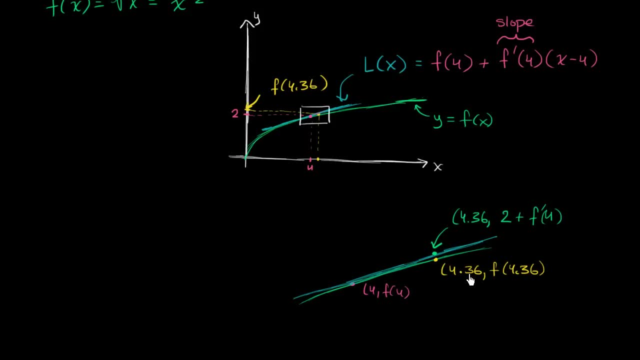 times x minus 4.. So 4.36 minus 4 is going to be times 0.36.. And that makes sense. You're starting at 2. And you're saying: okay, my change in x, my change in x is 4.36.. 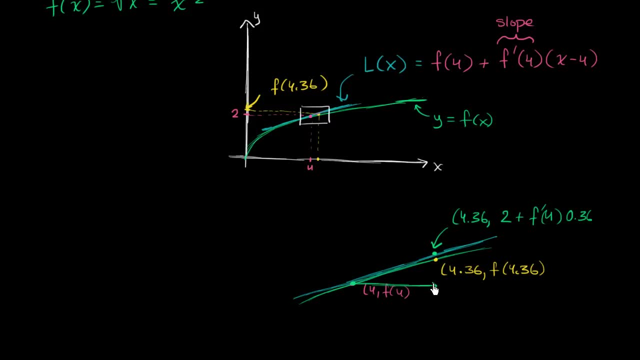 So my change in y is going to be my slope times, that change in x to get me that value, to get me that value right over there. So let's figure out, let's figure out what this, let's figure out what this thing. 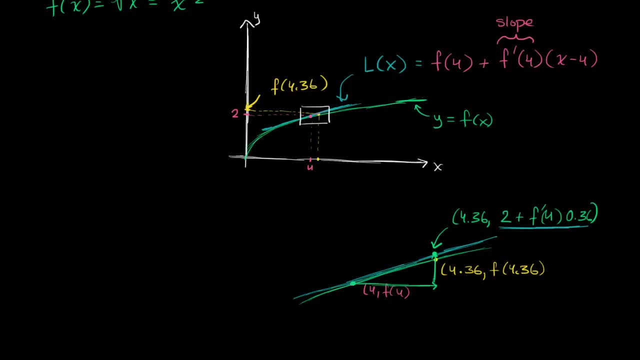 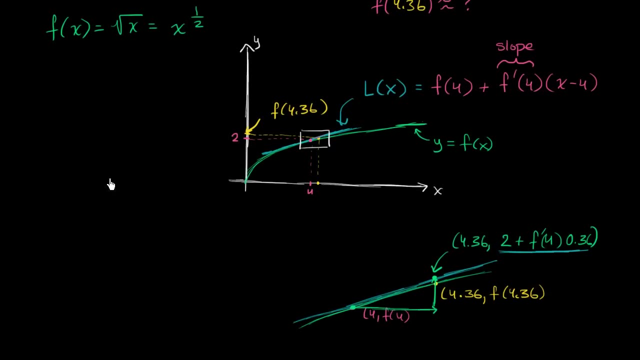 what this thing actually is. So to do that, we need to figure out f prime of 4.. So let's go back up here. I'll try to leave- actually I'll leave- this little visualization here. So let's see f prime. 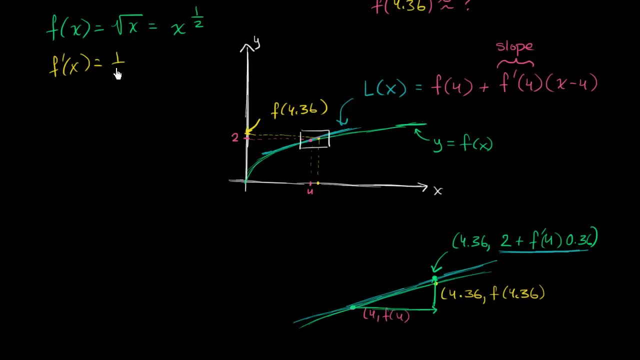 f prime of x is going to be 1 half x to the negative 1 half, just using the power rule over here. So f prime of 4, f prime of 4 is equal to 1 half times 4 to the negative 1 half. 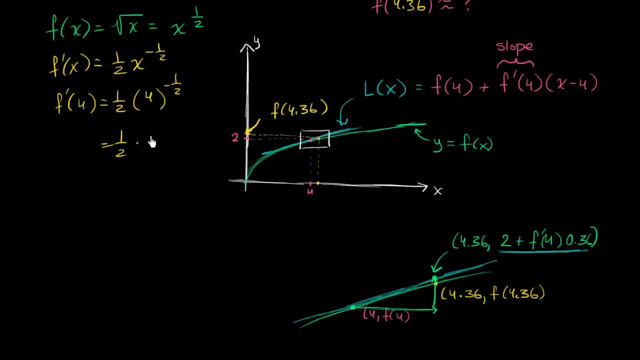 which is, of course, equal to 1 half times 1 half. 4 to the 1 half would be 2,, 4 to the negative. 1 half is going to be 1 half. So this is equal to 1. fourth, 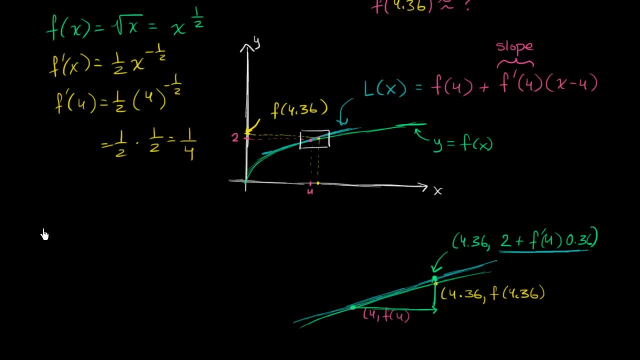 So l of we deserve a little bit of a drum roll now. l of 4.36 is equal to f of 4,. it's equal to f of 4, which is- let me just rewrite it- it's f of 4 plus f prime of 4. 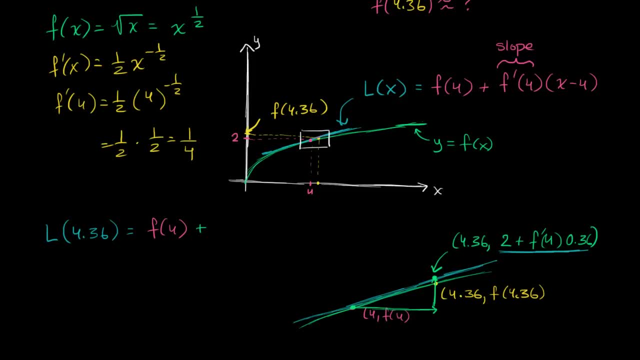 plus. gee, why am I switching to that color? Let me do the yellow Plus f prime of 4 times times times 4.36,, 4.36,. let me make this actually in a new color, just so we see it. 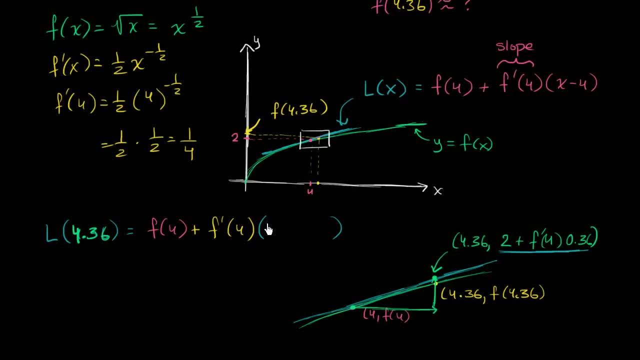 So 4.36, so times 4.36 minus 4, minus 4.. Actually, let me make all the 4's one color too, So you see it's the same. So just like that. So what is this going to be? 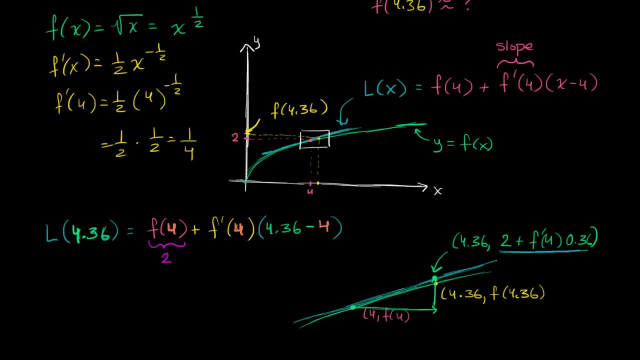 Well, this we already established is positive 2. This we already established. let me do this in the yellow color. this we already established is 1. fourth, and this part right over here is 0.36.. So this is going to be equal to. 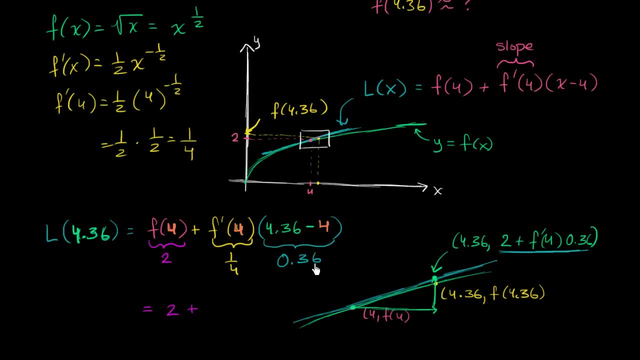 2 plus 1, fourth times 0.36 is 0.9, or 0.09.. So this is going to be equal to. this is going to be equal to 2.09.. So that is our approximation, And it should be. 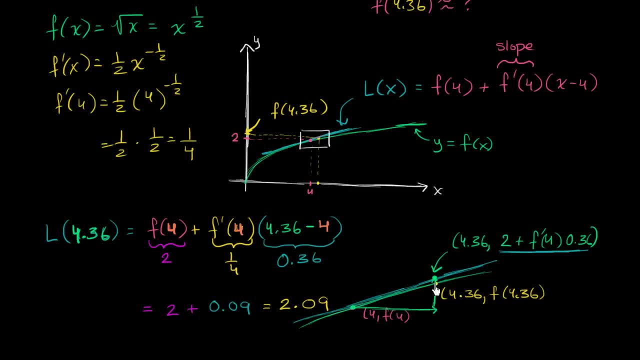 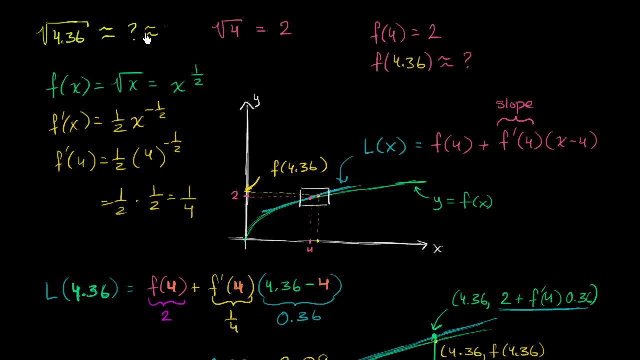 at least based on how I graphed it- a little bit higher than the actual value of the square root of 4.36.. But we could write that up here. This is going to be approximately. let me just write it this way.